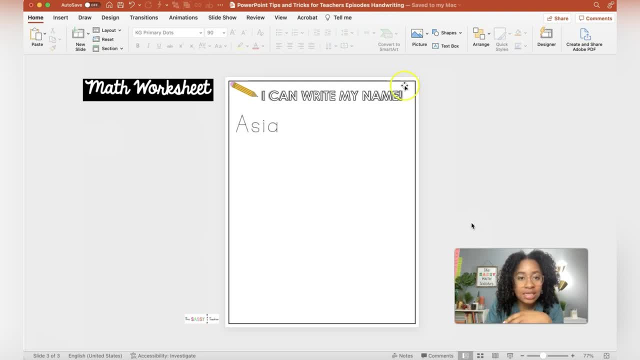 That way I can keep everything else. I'm just going to delete it. Okay, So that deleted all the lines, and now I'm going to delete my name. Okay, We're going to call this. Hmm, Let's do addition, Addition. I want it to be all caps again. 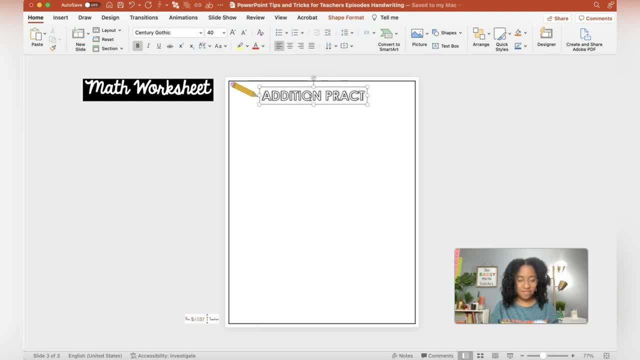 Addition practice: Fun, fun, fun Addition practice. Okay, So that's going to be the title And let's go ahead and dive in So say: you want your students to practice adding three numbers together. We're going to start by adding three numbers. So we're going to start by adding three. 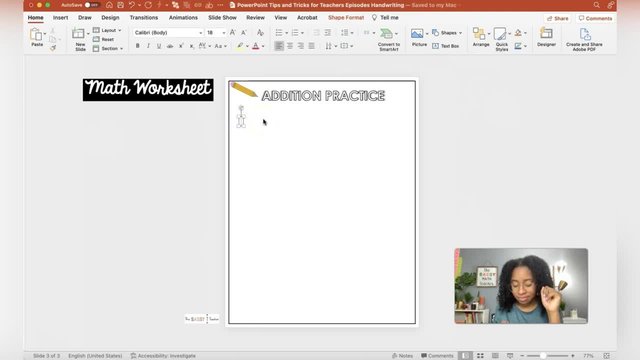 numbers, adding a text box and we're going to type our three numbers. So maybe it's 15,, 10 and nine. Ooh, not 69.. We don't want 69 in the classroom. Okay, My middle school teachers. 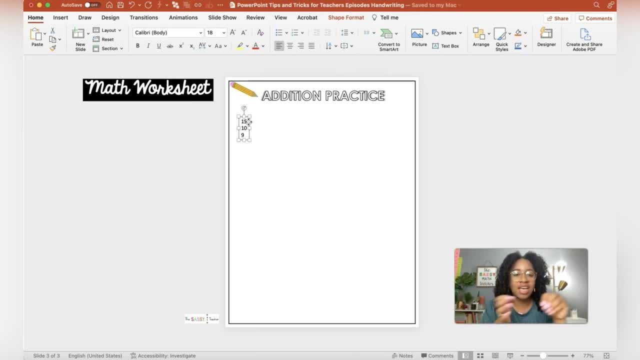 understand. Okay. So notice how these are, like, all justified to the left. I gave each number a new row, but what I do want to do is justify it to the right, And then, with this nine, I'm going to add a plus sign. So it's actually the basis of a math problem, Okay, So. 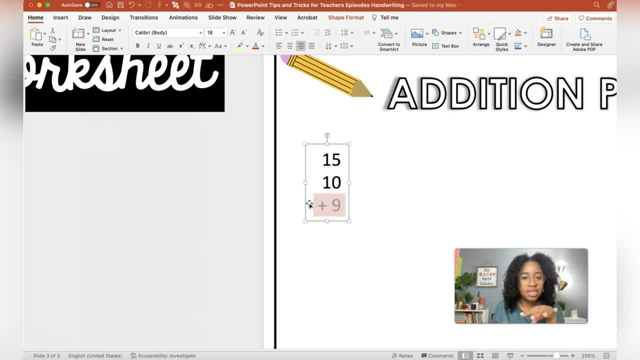 so we have that. now we want to have that little bar underneath, So you can do that in one of two ways. You can either just underline that bottom row to have it um, or you can physically draw out a line, Like we learned in the last couple of videos how to draw lines. Okay. 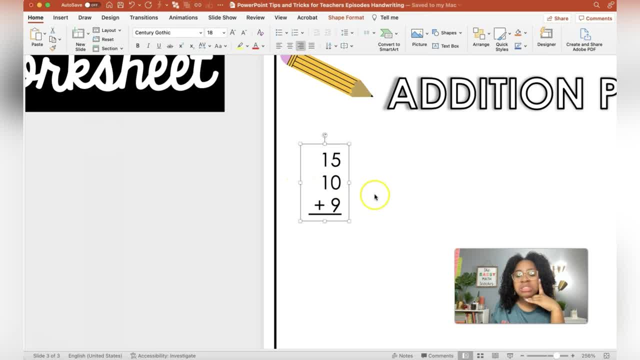 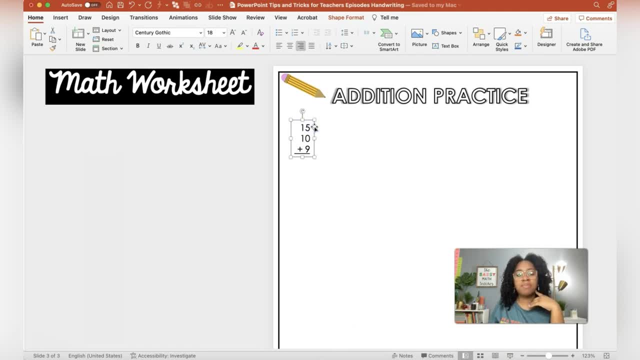 I'm going to go ahead and make this century Gothic because it's just a good, solid, free font that we can use. All right. So now we have that Um, but say you want it to be. you want it to be a little bigger, depending on what grade level you are teaching. You may want it to be a larger font. 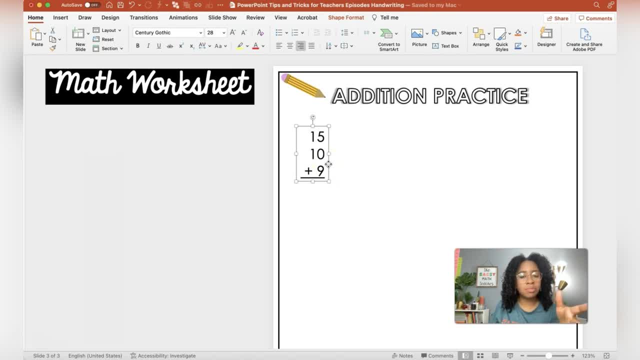 Depends, Um, but obviously we want more problems on a page. So what we're going to do is simply duplicate this one by doing command D and then space. We have, like I'm going to pick that out so you can do it- that close, So you can do it further. 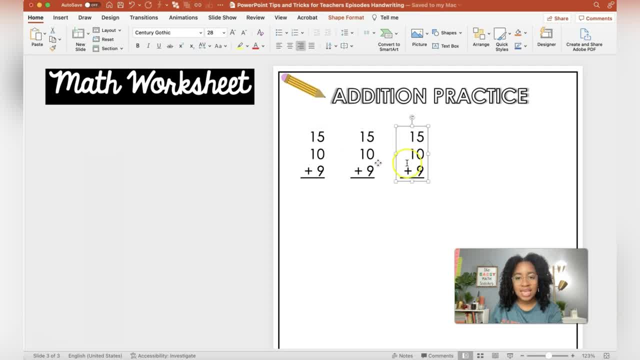 apart. I think I'm going to do it about there And then duplicate again. that way it will do it all the same distance. Okay, And you notice this one over to the right is going a little bit off of the page. That's okay. I'm just going to select all of them And with the arrows on my 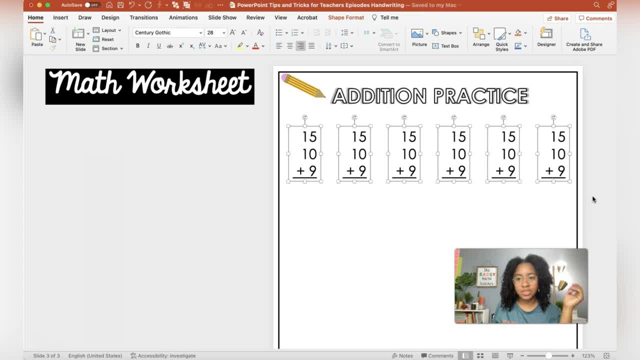 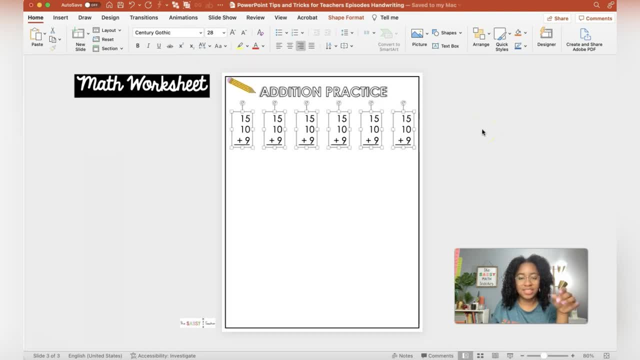 keyboard. I'm just going to scoot them over. That looks decent, Okay, Um, obviously we don't want our students to do the same over and over again, So we'll change the numbers in a little bit, But what I am going to do is go. 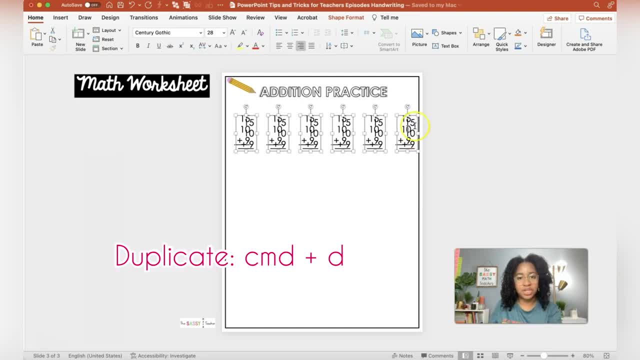 ahead and duplicate all. Notice, I have all six selected, So we're going to duplicate that again and just drag them about down here and just make sure they are also centered. Okay, that looks good to me. So now you would just go back through there and change all. 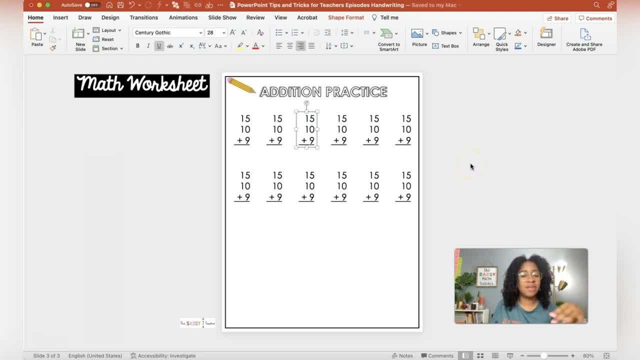 the numbers to fit your needs. whatever those needs may be, Okay, And maybe down here at the bottom you want something a little more challenging for them, So maybe I'm going to add another text box. You want to have something like 15 plus 10 plus, I don't know. So I'm going. 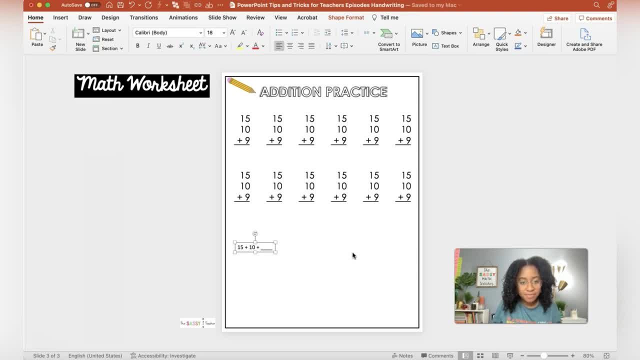 to do: shift with the underscore key and do a line and then equals Um 63.. Okay, Um, or actually 25 plus nine is 34.. So maybe that's what we should do. I wouldn't technically do that because it's right there on the page, But anyways. 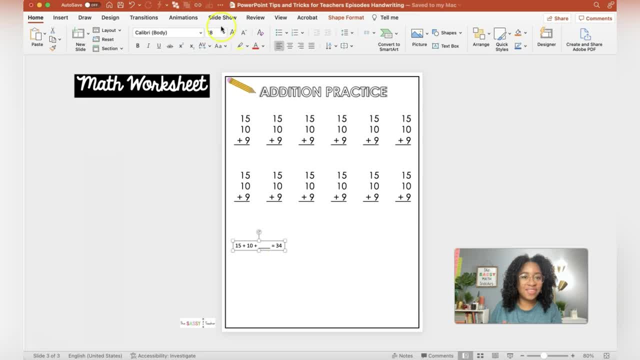 so maybe that's the next thing you want to do, where you have some questions where they had to fill in the blank. So what's missing? Um, but one thing you may want to do is actually separate the two halves of the page, So I'm going to go add a line in. 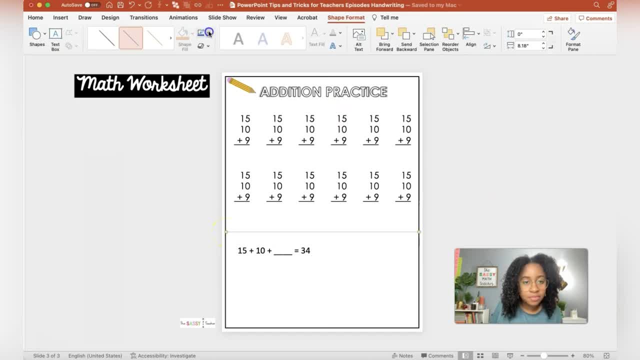 Just so it's kind of separated. Okay, All right. So the other thing that I didn't mention in the last video is that you need some directions on your paper. Um, actually, let's- before I forget, let's make that century Gothic. So you do need some directions and you may.